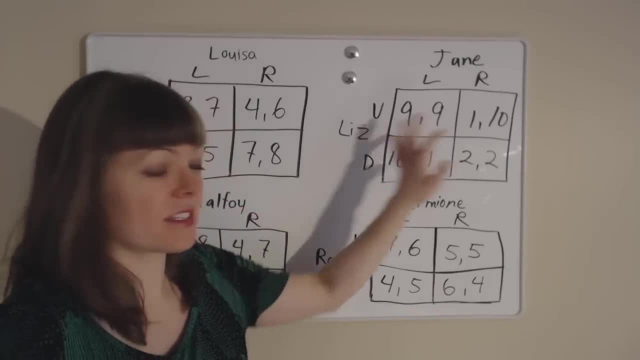 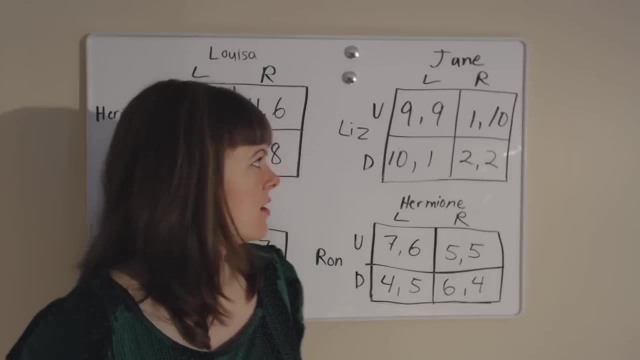 There can be four Nash equilibrium, for example, if everybody has the same payoffs. So we don't go into the problems with any preconceived notion of that. So let's get some practice, All right, And of course all my examples are from Jane Austen and Harry Potter. 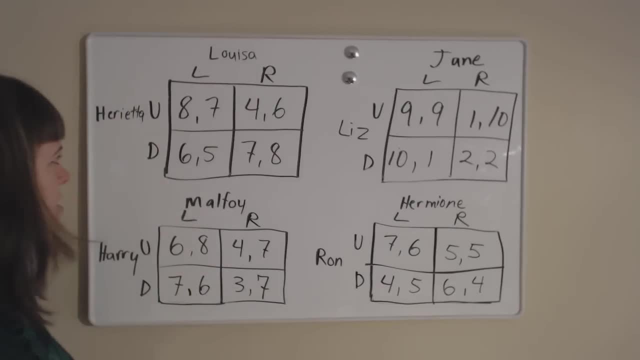 So we have Henrietta and Louisa from Persuasion, And Henrietta can go up and down And she is, of course, player one. Louisa can go left or right And she is player two. So, starting from Henrietta's perspective, 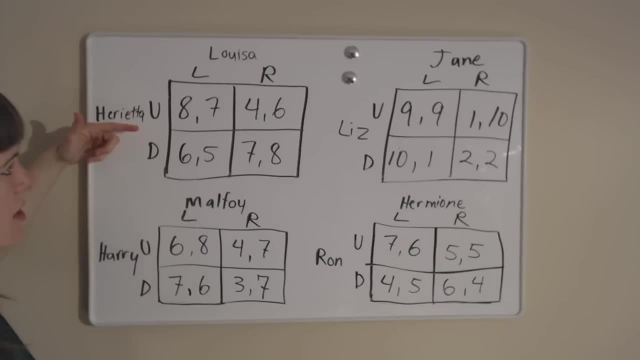 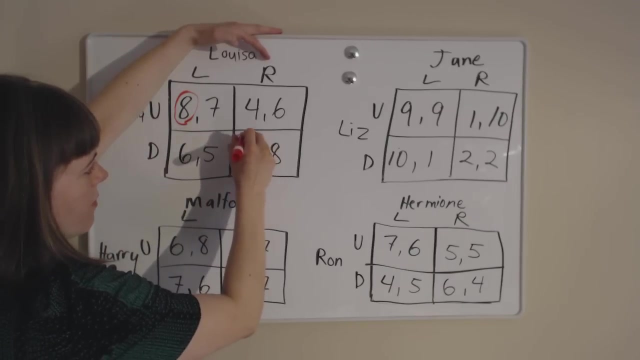 we're going to think about what Henrietta's best response will be to each of Louisa's strategies. So we're thinking Henrietta's perspective right now. So if Louisa chooses left, Henrietta prefers the eight over the six. If Louisa goes right, then Henrietta prefers the seven over the four. 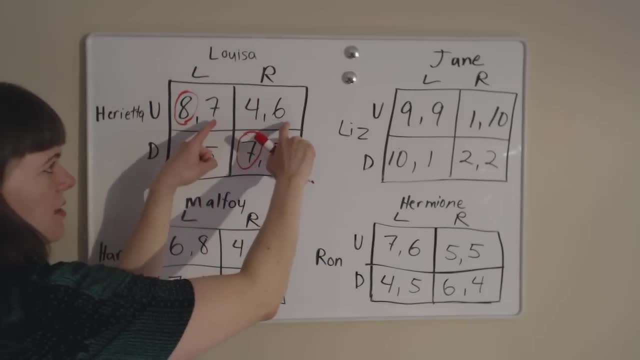 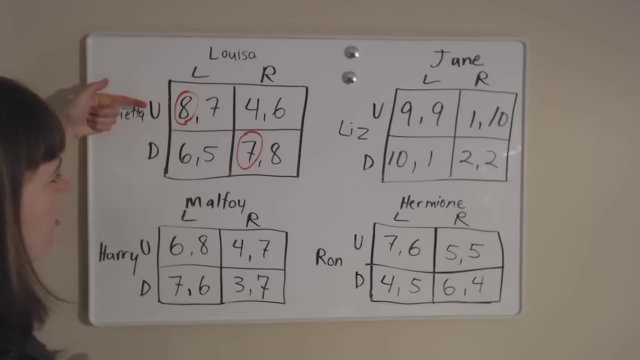 Now we switch perspectives and we're going to think from Louisa's perspective- player two- But we have to check Louisa's best response to each of Henrietta's strategies. So if Henrietta goes up, we're going to be liking the seven. 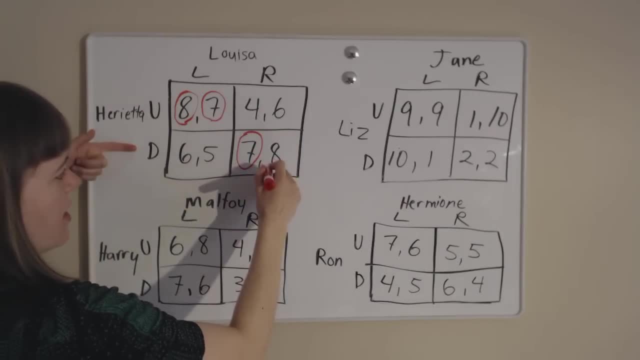 Better than the six. If Henrietta goes down, we like the eight better than the five. So in this case we have two Nash equilibriums. One is Henrietta going up, Louisa going left, The other is Henrietta going down and Louisa going right. 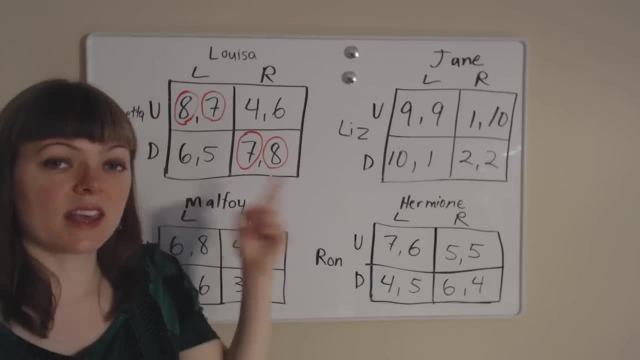 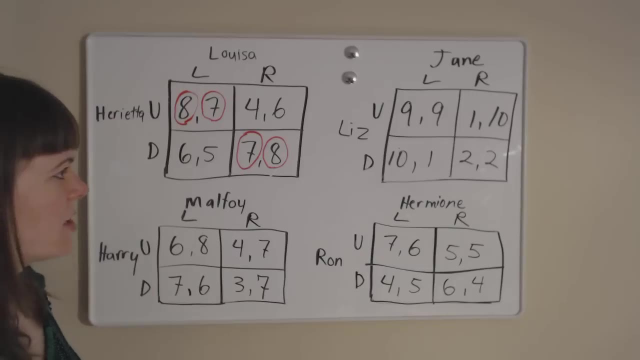 And in both of those perspectives each player can say: given if we end up down here, given what the other player did, I'm happy with my choice. So two Nash equilibriums there. So let's come over to Liz and Jane from Pride and Prejudice. 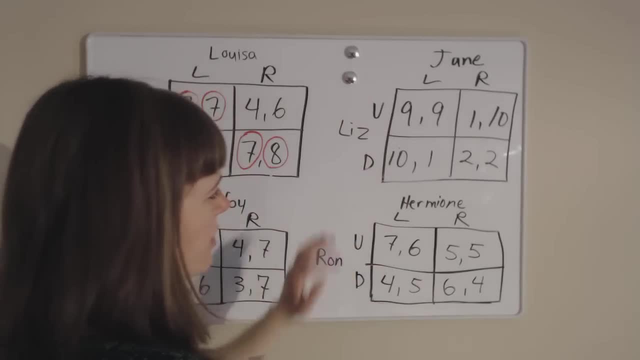 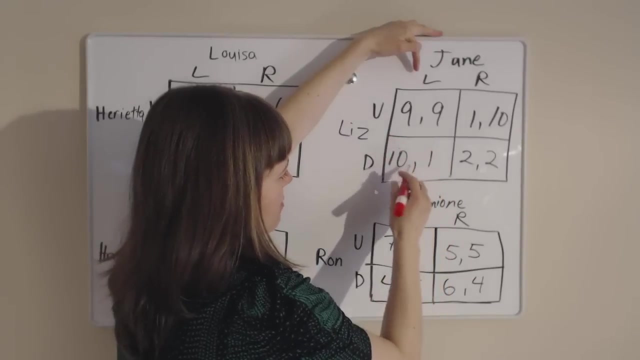 All these players have the same strategies up and down, left and right. So we'll start from Liz's perspective, meaning player one, And we want to check Liz's best response to each of Jane's strategies. So if Jane goes left, Liz likes the ten better than the nine. 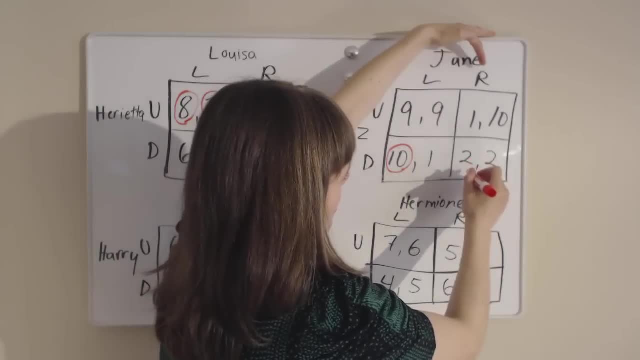 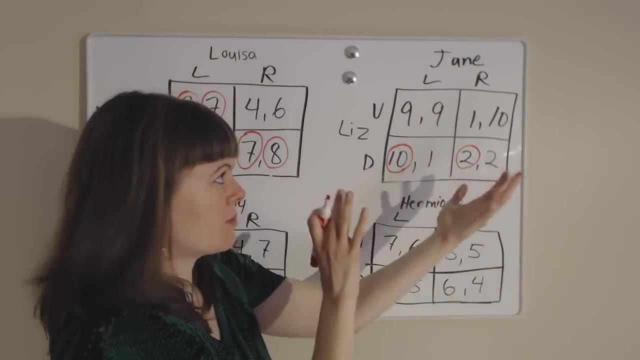 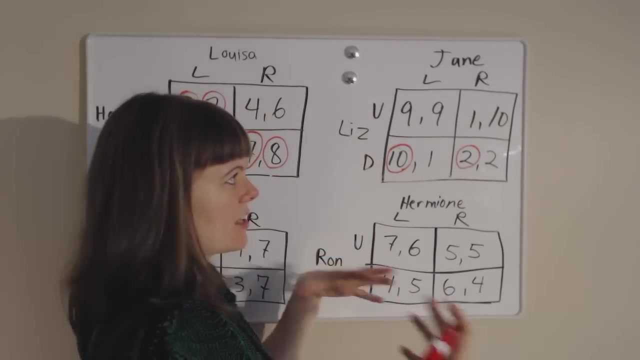 If Liz goes right, Jane likes the sorry. if Jane goes right, Liz likes the two better than the one. And now we switch perspectives and we're going to be thinking from Jane's perspective, meaning we're looking at player two's payoffs and we're going to check Jane's best response to each of Liz's strategies. 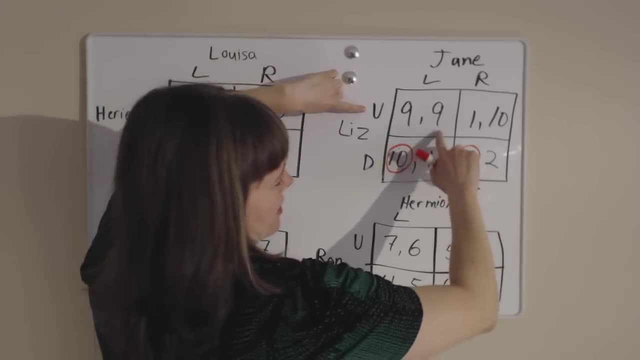 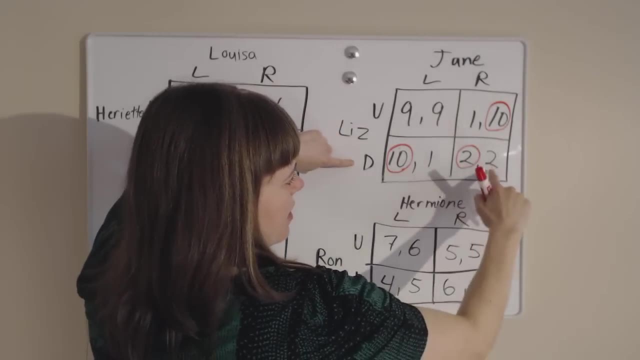 So if Liz goes up, Jane's best response is going to be to choose the ten, And if Liz goes down, Jane's best response is going to be to choose the two. So here we have our Nash equilibrium, and this is actually a prisoner's dilemma. 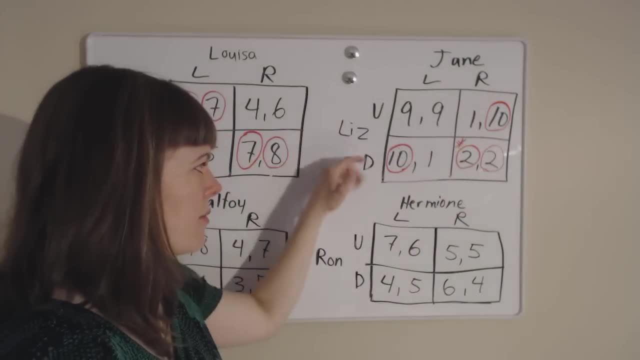 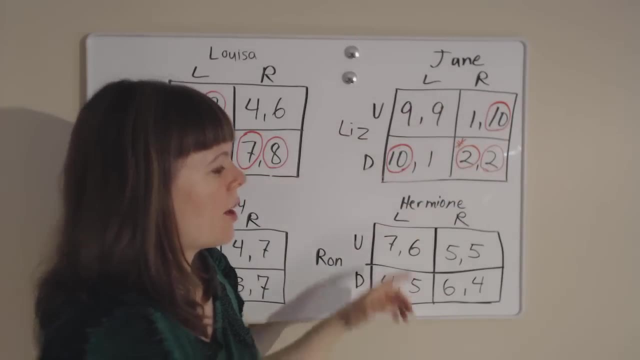 Both players have a dominant strategy. Jane's dominant strategy is to always go down. Liz's strategy is to always go down. Jane's strategy is to always go right. But when they get there, they both would have preferred the situation where they both chose their dominated strategy. 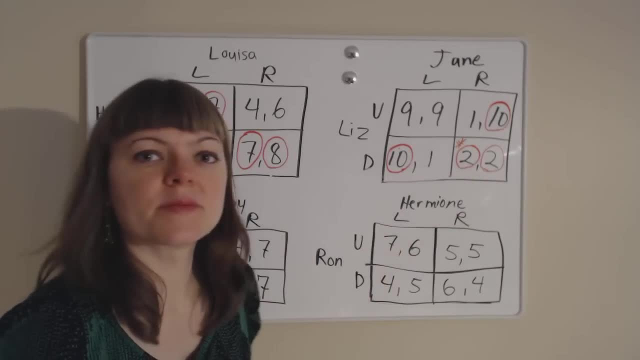 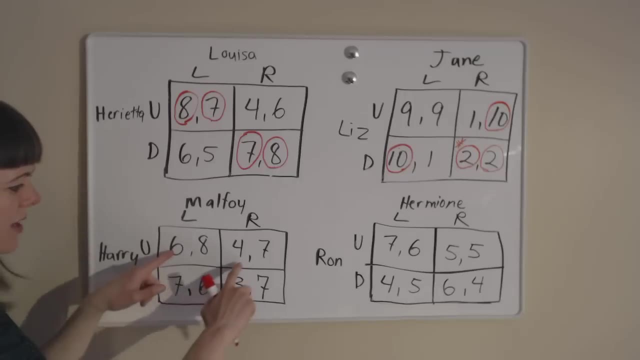 And any time you have that. it's a prisoner's dilemma. So let's try Harry and Malfoy. We have this and we'll start in Harry's perspective, meaning we're looking at player one's payoffs. We'll check Malfoy's strategies from Harry's perspective. 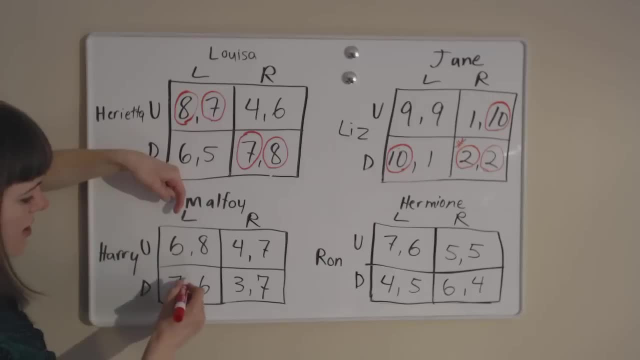 So if Malfoy goes left, Harry would have wished he would have gone down and gotten the seven. If Malfoy chooses right, Harry would have wished he would have chosen the four. We'll switch perspectives and think about this from Malfoy's perspective. 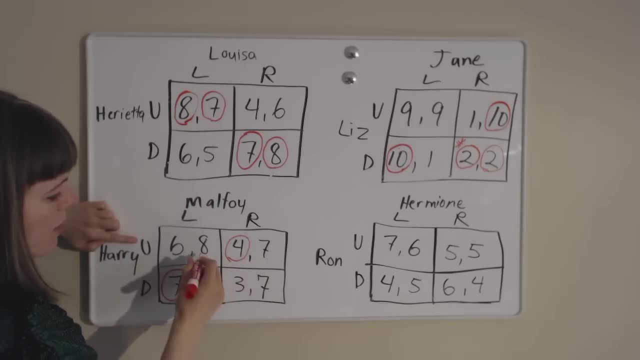 If Harry goes up, Malfoy would have wished he would have chosen the eight. He would have wished he'd gone left. If Harry goes down, Malfoy's perspective, His best response to Harry going down is to choose right. So in this game there's no match equilibrium. 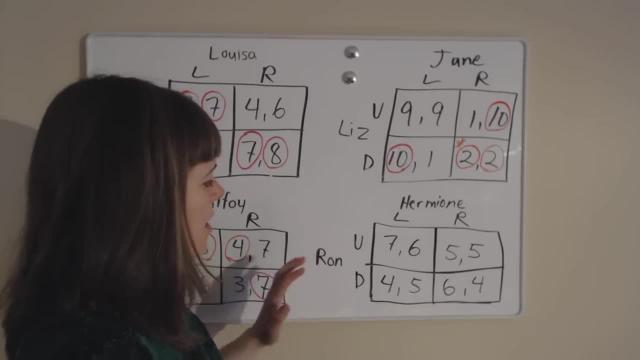 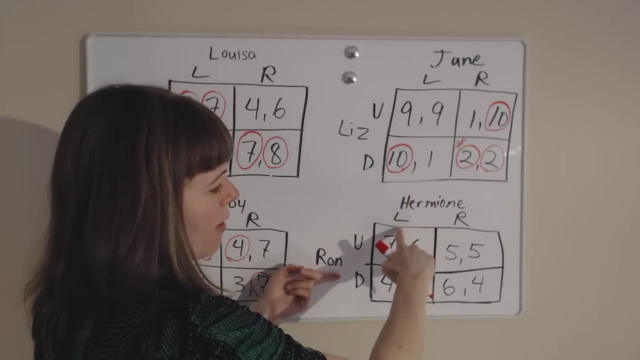 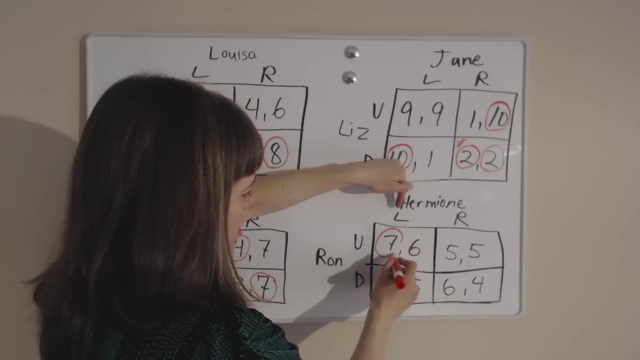 Over here we have Ron and Hermione playing a game and we'll start with Ron's perspective. So if Ron goes up- sorry, Ron's perspective meaning we're going to check Hermione's strategies. So if Hermione goes left, Ron is choosing between the seven and the four.